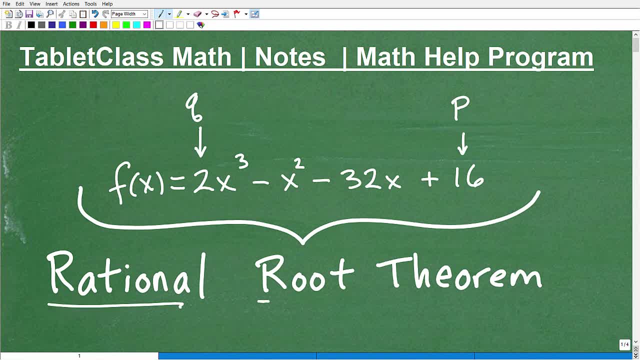 Okay, let's talk about the rational root theorem. And this is an extremely important theorem in mathematics and specifically algebra, And it has to do with solving polynomial equations. So if we take a look at this particular function, this is a polynomial function, It's a third degree polynomial function. So if the objective here is to find the solutions, find the zeros roots, those are all. 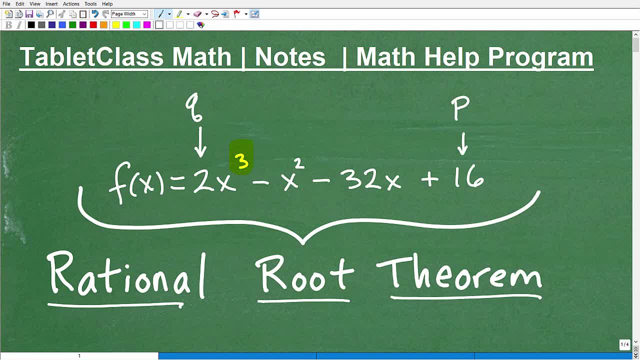 different terms. I mean basically the same thing means take this equation, this function, as polynomial function, set it equal to zero and solve for x, right? So that's what we're trying to do here, And the rational root theorem is going to assist us in this objective. Okay, but before you kind of study the rational roots, you need to already have a pretty strong background in solving polynomial equations. First of all, you need to know a few things before. 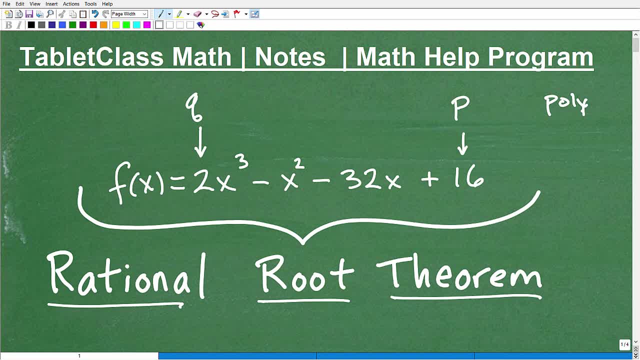 we kind of get into this video. One, what is a polynomial? And another thing would be useful is: what is a rational root? Okay, what is a rational root? And this is quickly cover some, some basic concepts that hopefully you already understand. If you don't quite know what I'm talking about, please continue to watch the video. I think you'll. you're definitely going to benefit from, but benefit from it, But you'll. it's an indicator that you need to do some review, Okay. 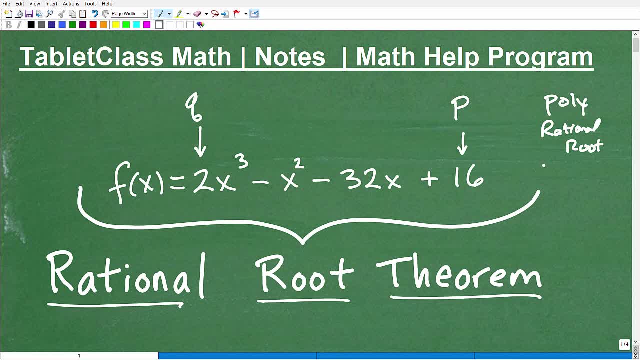 All right. so first things first. So let's think about an equation like this: 2x plus one equals nine. how many solutions is to this linear equation? this happens to be a polynomial equation to the first power. there's just one solution. Okay. how about this? x squared equals 16.. This is a second degree polynomial equation. we call these guys what quadratic equations. there are two solutions, Okay. So, for example, 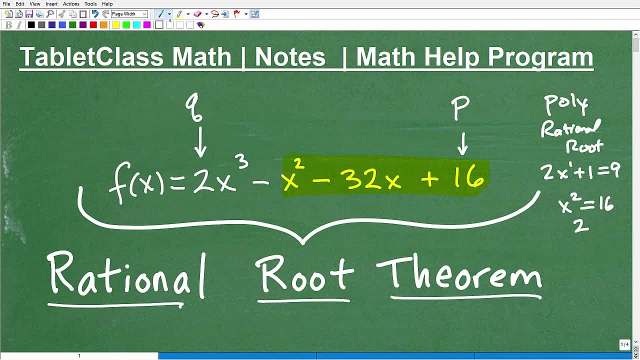 here. if I said: take this part of this equation, this polynomial equation- let's forget this for a second- and set it equal to zero. how can I solve this quadratic equation? Well, a quadratic equation is a degree two- polynomial- Okay. So I'm thinking to myself: well, how many solutions is there? There's two solutions. there's always two solutions to a quadratic equation. Well, how can I find them? Well, I'd like to be able to, let's say, maybe factor this. that'd be great. But if I can't factor a, 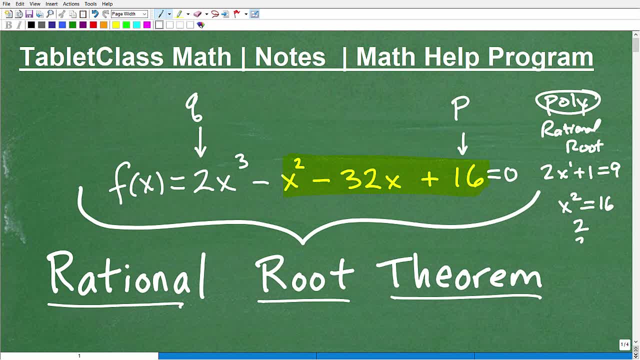 quadratic equation or a degree two polynomial. I can always break out my trusty friend, the quadratic formula, and that can handle any situation right. So I can just take my quadratic formula, apply it to whatever degree two polynomial equation I have and I will get my solutions. 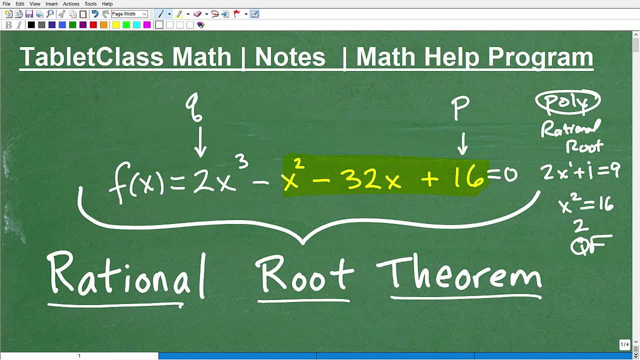 So when we're talking about polynomials, you know solving degree one and degree two polynomials we can. you know there's direct paths, we can always get the answer. But things get more interesting when we have a third degree polynomial or higher. So, like this particular problem, 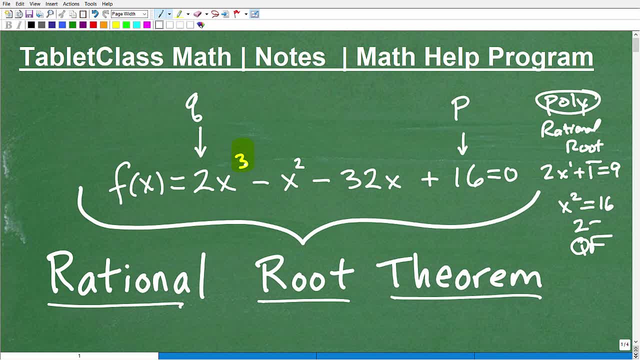 there is no quadratic formula for degree three. you know polynomial. we can't just plug this stuff into some formula. I get the answer. So we need additional tools, we need new tools, okay, So we need to already know how to solve quadratic equations on obviously a lot of your questions. 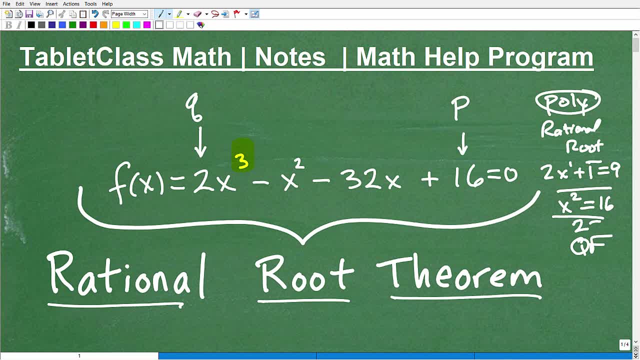 we need to know how to do this, But, above and beyond that, we're going to need some more advanced- you know math methods to be able to solve this polynomial equation, And that is indeed rat. the rational root theorem is one of those methods that we need to understand. Okay, so, again, you should have a 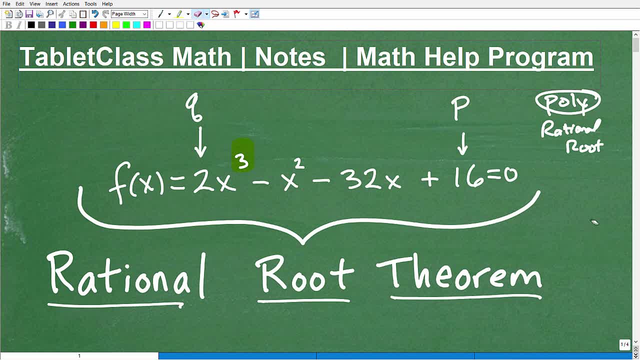 good, strong background in solving quadratic equations And understanding basically the fundamental theorem of algebra which states that if I have a polynomial equation, the degree of that equation okay. so this is a third degree. polynomial right is real número or imaginary or complex number solutions? We just don't know until we get into this problem solving Okay. 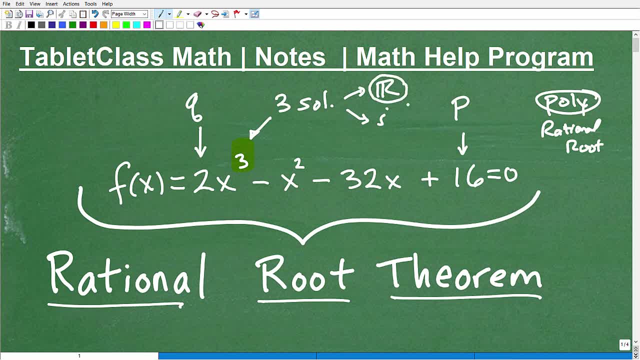 Now part of the real number system. okay, one type of number is rational roots. So rational roots are numbers that you can. you'll think of them as integer values. let's say like negative 3,, 2,, 1, okay, but technically, rational roots are numbers that we can express as fractions of. 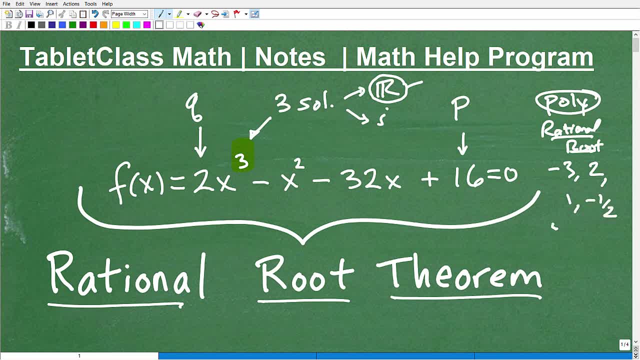 integers, so like negative 1 half, okay, or 2 thirds or 7 tenths, okay. these are numbers that we can, any fractions that, where the numerator and denominator are integer values, whether they be positive or negative, all these numbers together are rational roots, okay, so obviously. 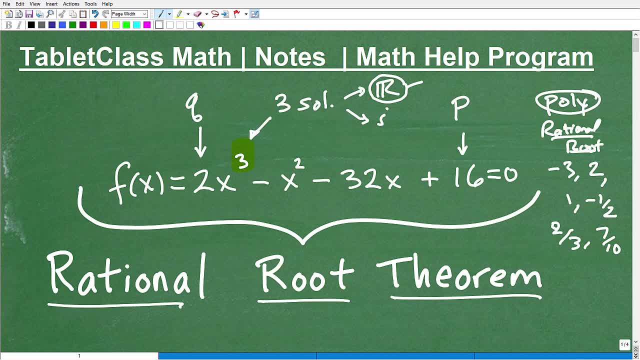 the rational root theorem has something to do with rational numbers. okay. so, with all that kind of being said, I'm going to get into the direct application of the rational root theorem here in a second. but it's important to have this foundational, you know, background information. 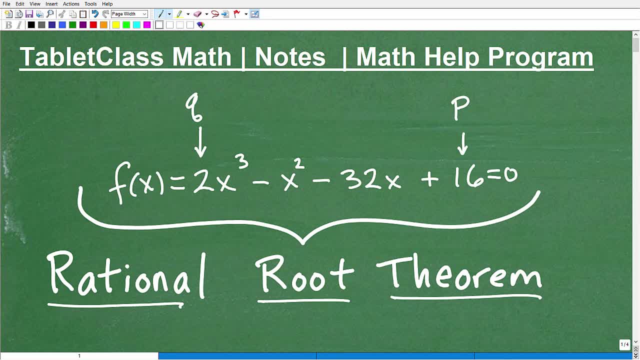 because if you didn't understand what I just got done talking about, then this might be a little bit more complicated than you might think. okay, it's not overly complicated, you could still understand this, but you know, in terms of you know, you mastering this, you got to master the. 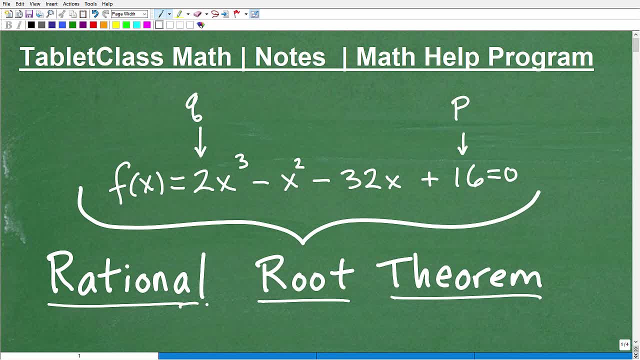 other stuff that we just talked about before. you can master the rational root theorem okay. so I want to get all that in a second, but let me first quickly introduce myself. my name is John. I'm the founder of Tablet Class Math. I'm also a middle and high school math teacher and over the 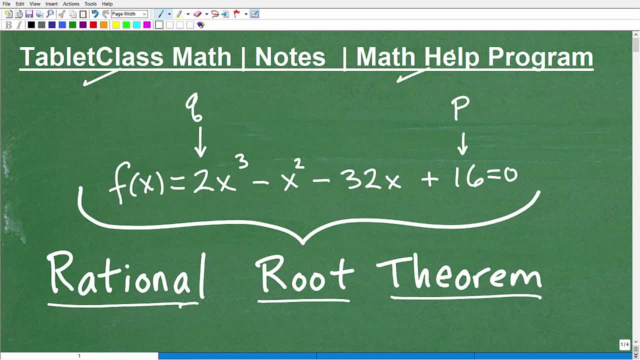 years, I've constructed what I've what I believe is one of the best online video-based math help programs in the world, and I've been doing a lot of research on this and I've been doing a lot of work on this. and I've been doing a lot of research on this and I've been doing a lot of research on this. 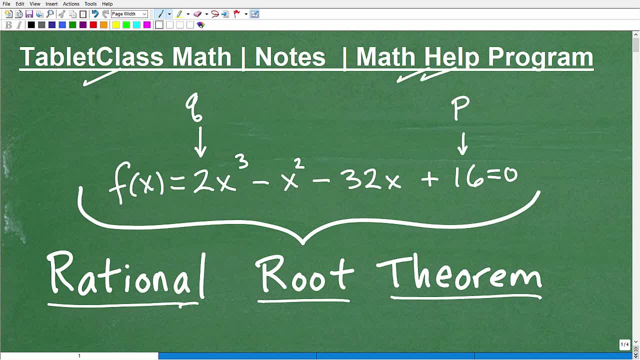 there is. so whether you need to take a full, comprehensive, a complete math course, I offer that- or you need assistance with a course that you're taking right now. I can help you out. all right, so you can find a link to my math help program in the description of this video. 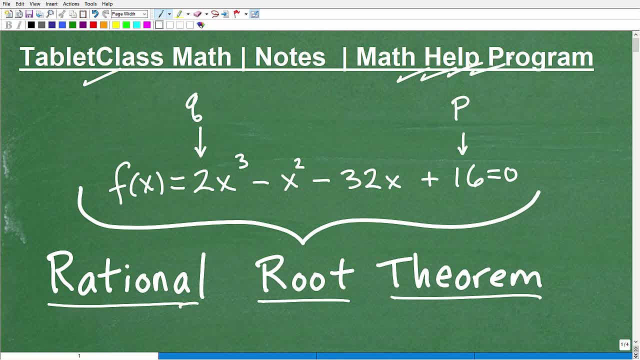 those will include full, comprehensive, very detailed lessons on all the topics you know you're basically with the middle and high school mathematics and I teach you how to solve the most common math problems that you're going to find at those levels of mathematics. 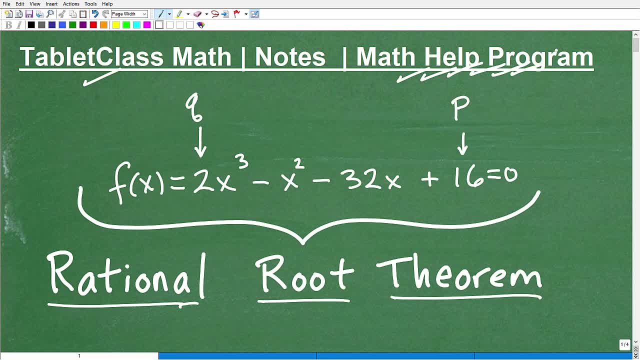 I teach you how to solve the most common math problems that you're going to find at those levels. I literally solve thousands of problems, all video based, So a really great program that's taken me years to build, But I'll let you be the judge of it. If you're interested, you can find it in the link in the description. 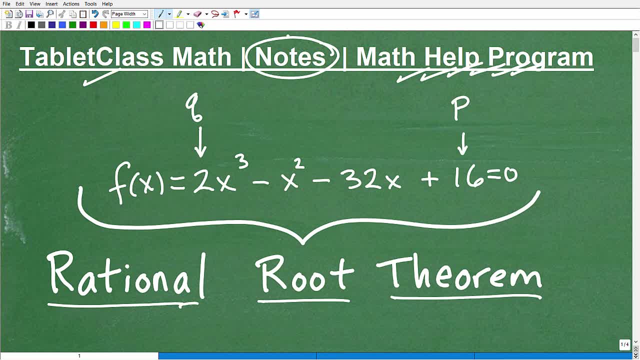 Now, as a math teacher of teaching for decades, there's one thing that I need to stress to you is math notes. OK, it's just as a general golden rule of math. that I've seen is those students who take great math notes typically have great math grades. 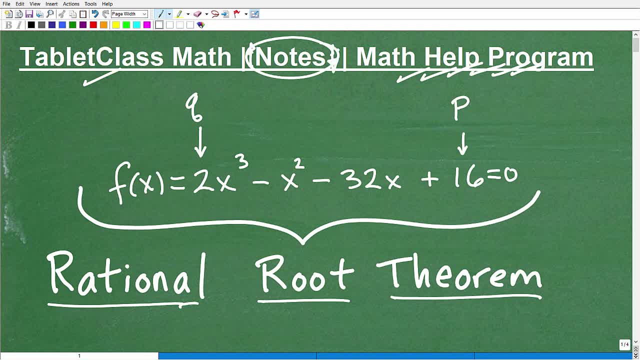 And the reverse is true: Those students with no notes, sloppy math notes. maybe their dog ate their homework and their math notes? Whatever the case is, take a look at your notes. OK, make an honest assessment. All of us have room for improvement. 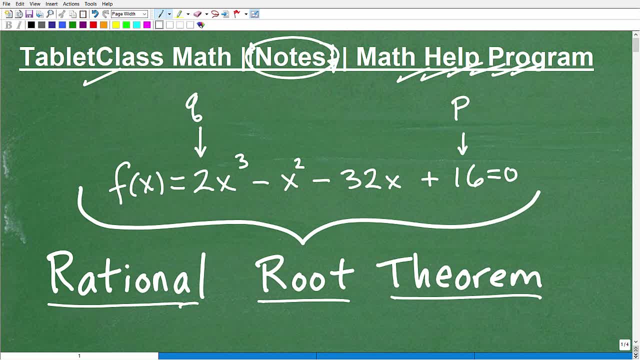 Very, very few people take perfect math notes. But yet if you're really struggling in this area, that's your first starting point to really improve in mathematics. But in the meantime you need something to study from. So I actually offer very detailed, comprehensive math notes. 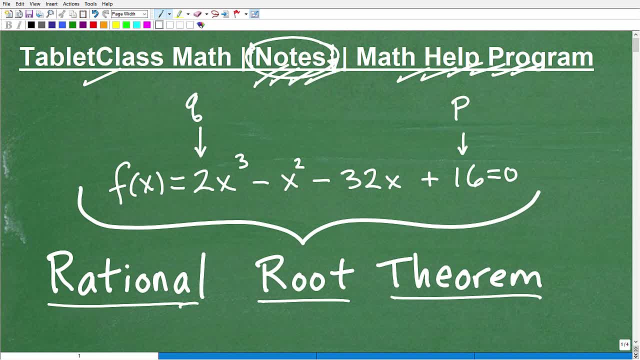 Those will include pre-algebra, algebra one, geometry, algebra two and trigonometry. For the rational root theorem, you'll want to check out my algebra two trig notes. OK, let's get into the rational root theorem Again. I just laid out, as an introduction to this video, what we're talking about. 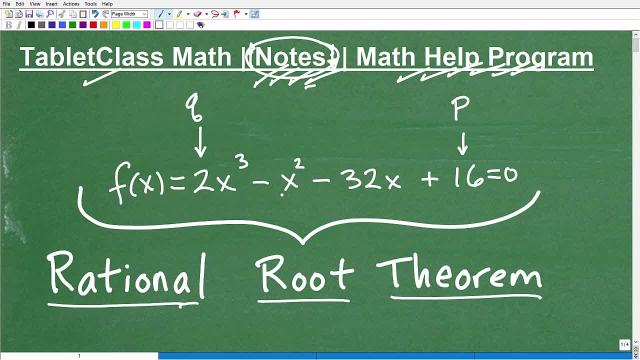 The objective here is to solve this. It's a third degree polynomial equation. So, by the way, the rational root theorem could apply to quadratic equations as well, But we don't really need to apply it because we already have the quadratic formula. 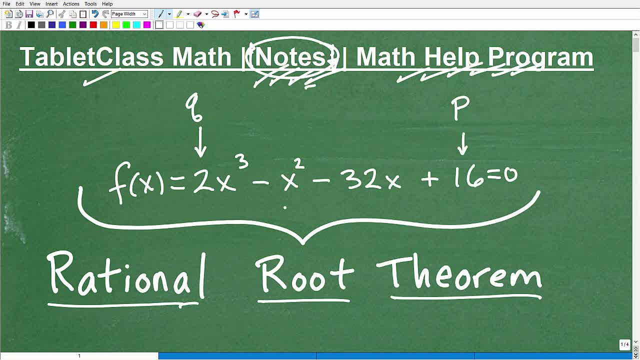 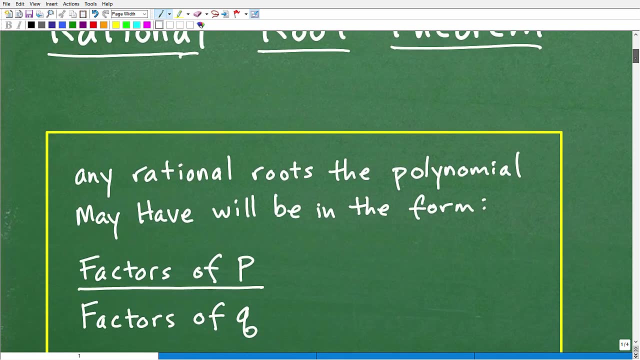 But there's. it's not really necessary, But the objective is: how do we solve third degree or larger polynomial equations? We need new, advanced tools, Obviously the rational root theorem being one of them. OK, so here is a quick overview of what it is. 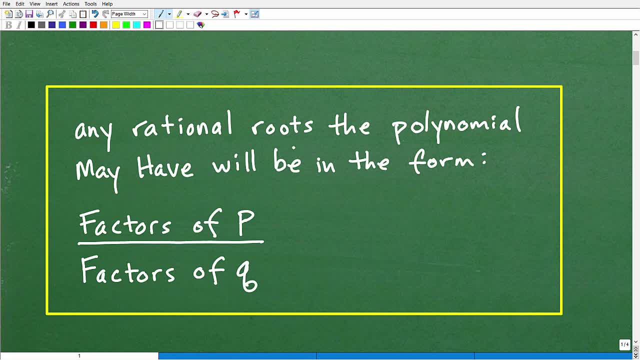 And basically the rational root theorem states that any rational roots the polynomial may have. OK, there's no guarantee that the polynomial is going to have rational roots. OK, we already described what rational roots are. They're like numbers, like two negative three, one half negative, two fifths, whatever the case is. 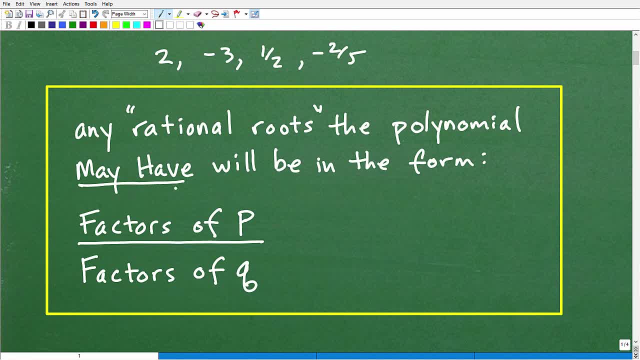 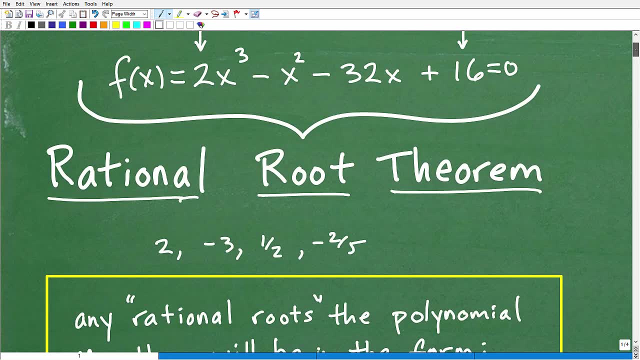 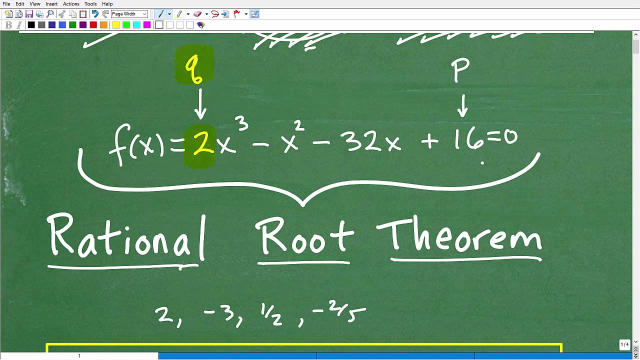 But here's the thing: If any rational roots the polynomial may have, will be in the form of the factors of p over the factors of q. And what is p and q? So up here? OK, q is the leading coefficient. So notice that my polynomial is written in standard form. 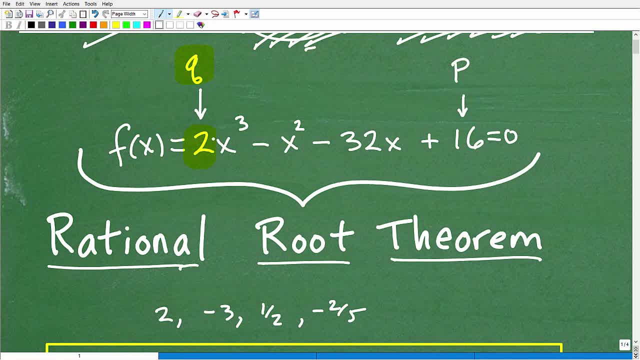 When you write a polynomial from the highest power to the lowest power, your leading coefficient here is q. OK, and your last term, your constant term here of the polynomial, the number OK, if you will, is p. OK, so we're going to look at the factors of p and the factors of q, the leading coefficient and the last number. 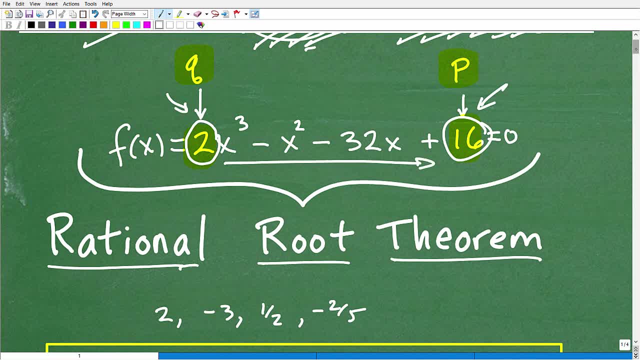 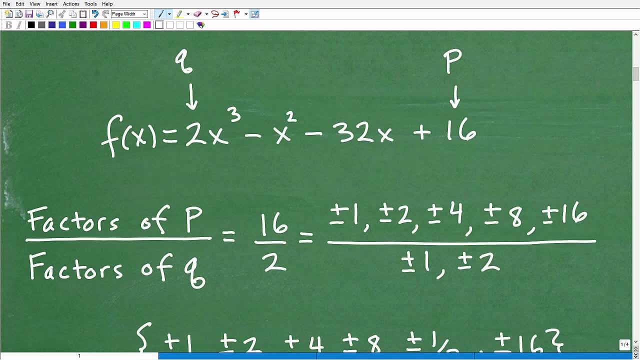 of the polynomial when it's written in standard form. OK, so we're going to go ahead and do that now, And then we'll see how we actually use this information. OK, so here's q And here's p. OK, so what's the factors of p? 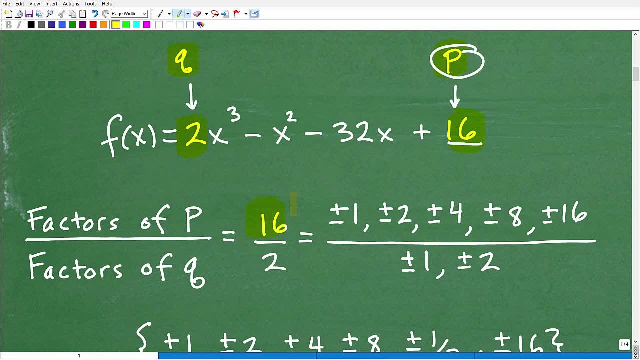 Well, p is 16.. OK, so we're going to- I'm going to talk about all this here in a second, And then we have the factors of q. So q is two, All right, OK, so let's talk about 16.. What are the factors of 16?? 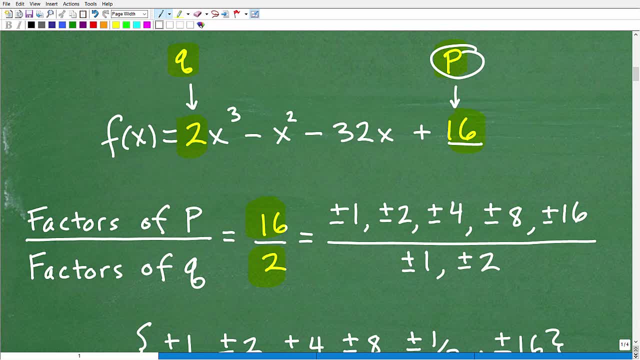 Now these are the factors of 16.. But let me explain this for a second. The way I'm doing this here is the way you want to do this in practical application with the rational root theorem. So 16,, let's say, for example, is equal to 1 times 16.. 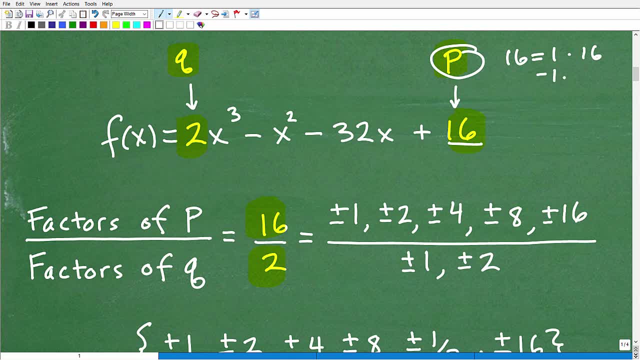 Positive 1 times positive 16 is 16.. And negative 1 times negative 16 is also positive 16.. So 1 and negative 1 are factors of 16.. So I'm going to write that as plus or minus 1.. There's no need to write 1 and negative 1.. 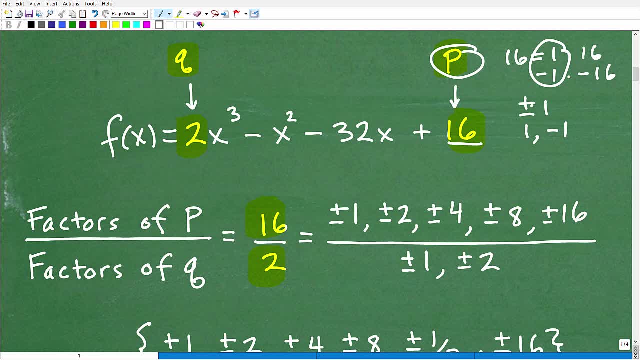 OK, we can just write it as plus or minus 1.. So the way you want to list the factors of your numbers- let's take 16 here, for example- is you're going to go from? you're going to always start with 1. 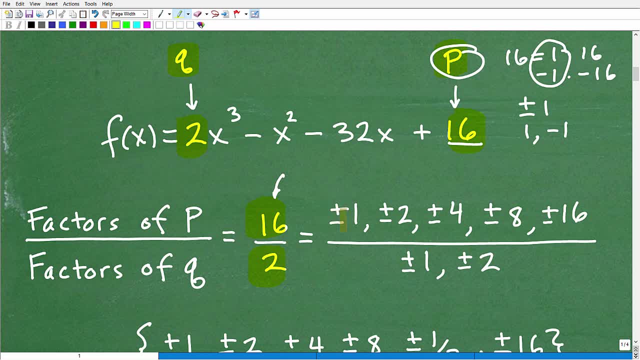 and you're always going to have a plus or minus. You don't have to think about this. It's always going to be a plus or minus, So let's just think about it, All right? One is always going to be a factor of any number. 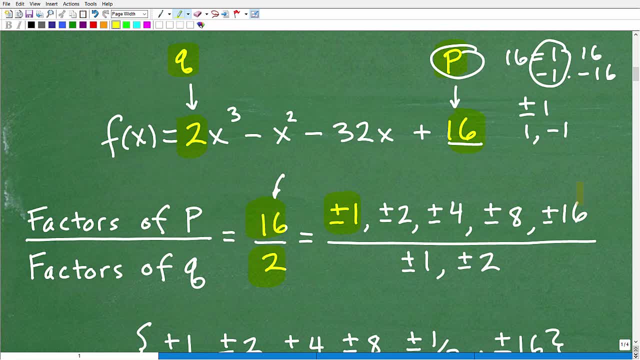 And, of course, 16 is a factor of itself. So that's going to be our last number. We're going to start small And we're going to work our way up to 16.. OK, start with the smallest numbers and work your way up. 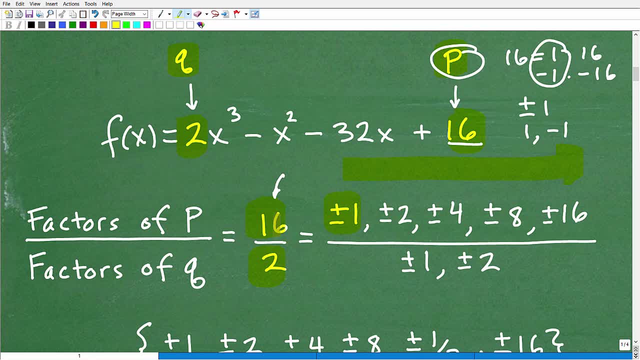 So just think to yourself: OK, what's the next smallest number? That's a factor of 16.. Oh yeah, 2 times 8 is 16. So that's going to be positive, negative, 2.. Then you start thinking 3 and 4.. 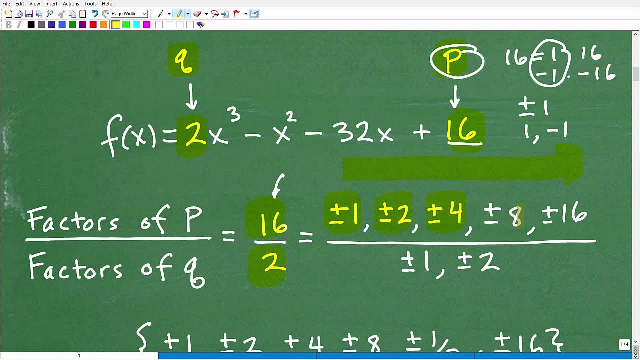 Yep: 4 times 4 is 16.. So that's positive, negative 4, 8.. OK, so the next one: 8 times 2 is 16, positive, negative 8. And then we have positive, negative 16.. 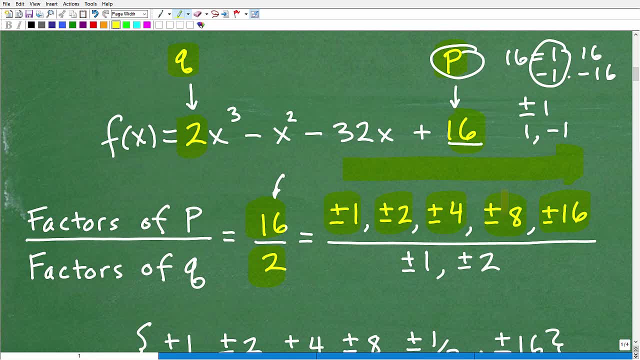 Always positive and negative. Always write it just the way I'm doing it, like this, OK. So factors of 2, remember: 1 is always your first factor: positive, negative, 1.. And then, of course, 2 is our last factor of 2, positive, negative, 2.. 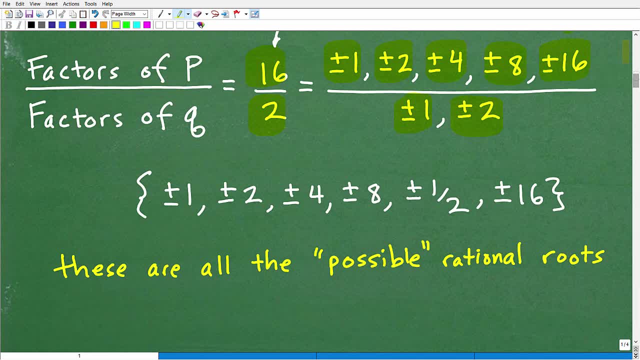 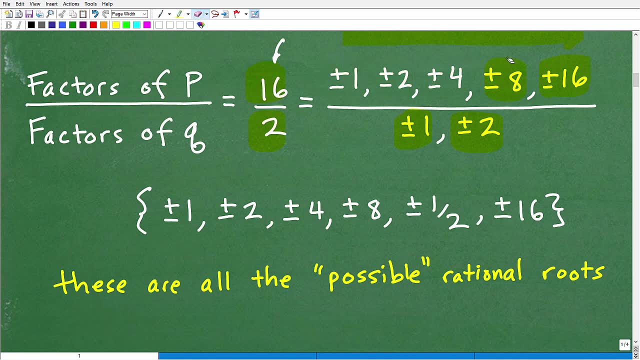 Now, once you have all your factors listed, OK, the next step is the following: OK, this is where students often get confused with this. All right, We're going to take one of the denominators We have to form. we have to list all the combination of numbers we can make out of. 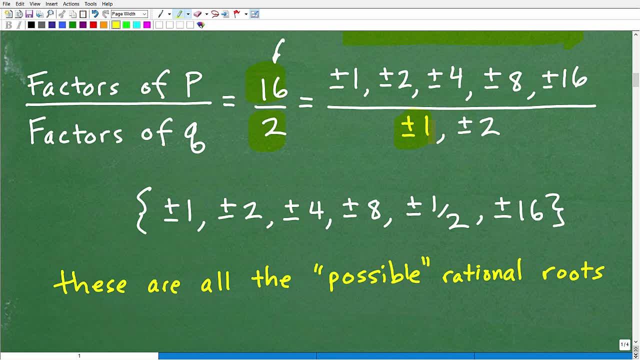 these various factors combinations. So this is the way you do it in practicality. We're going to take the first denominator, It's going to be 1.. OK, And we're going to divide it into all of our possible numerators. 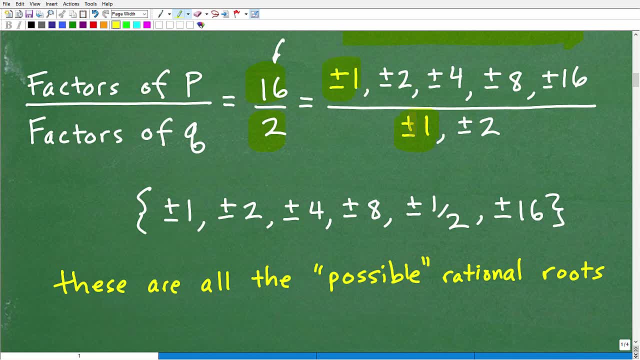 OK, so now for when you're doing this, just forget the positive, negative mentally in your head. Let's just look at the number, OK. So in other words, 1 divided by 1.. I don't need to go positive, negative, 1 divided by a positive, negative, 1.. 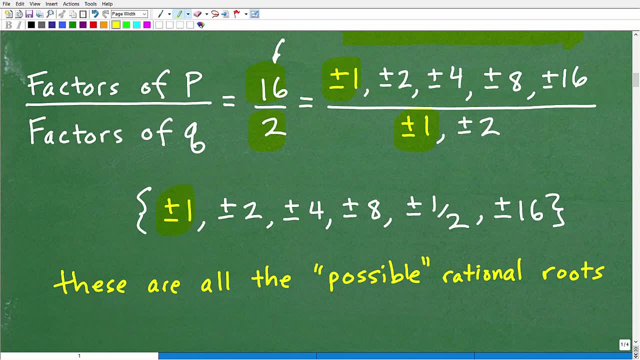 Just mentally, let's just go: 1 divided by 1 is what That's, 1. OK, 2 divided by 1 is 2. OK. now when you write your list here, you definitely need to put the positive, negative down there. 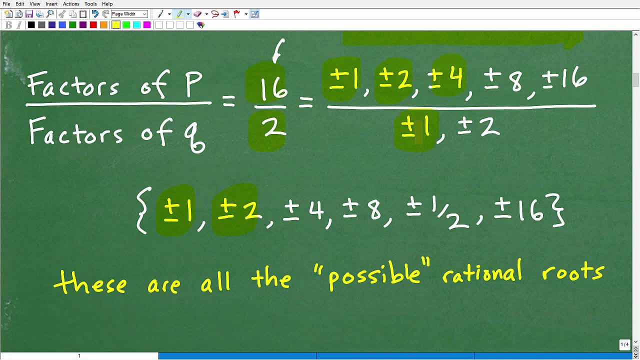 But we're just making these combinations: 4 divided by 1,, of course, is 4.. 8 divided by 1 is 8.. 16 divided by 1 is 16.. OK, so you're going to list all your numbers down there. 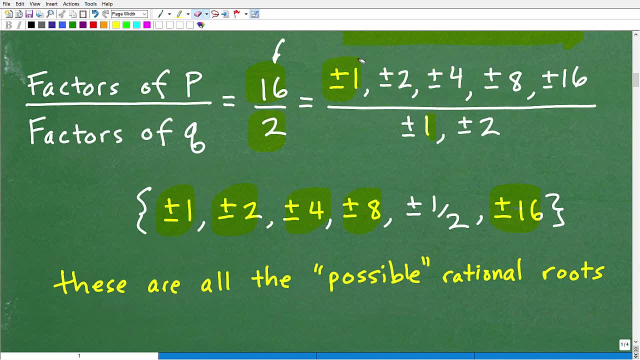 Then what we're going to do is we're going to now switch to the other factor, the next factor in the denominator. OK, so now there might be more. This is like positive negative 1, positive negative 2.. But maybe there's like positive negative 3.. 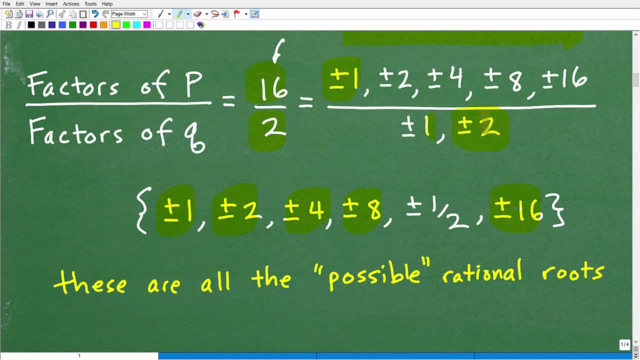 OK and some problem that might be doing. So we're just going to go to the next factor in the denominator and start looking at the different combinations and add it to our list. So we have positive, negative 1 or 1 divided by 2 is what. 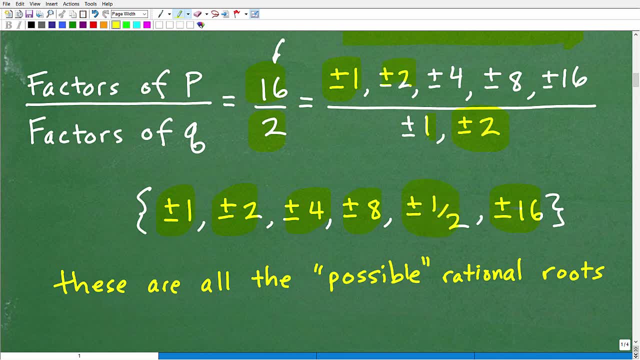 1 half, So that's got to be in our list here Now. 2 divided by 2 is what? That's, just 1.. That's already in my list. 4 divided by 2 is 2, that's in my list. 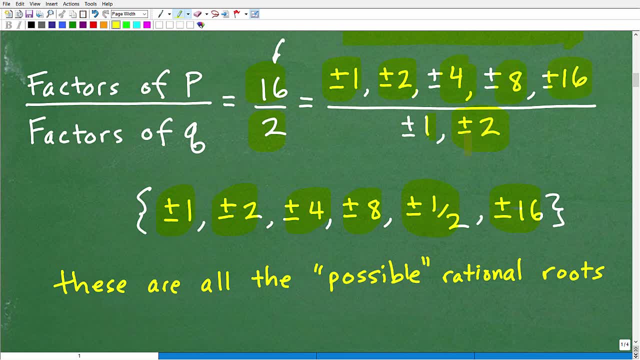 8 divided by 2 is 4, that's in my list. And then 16 divided by 2 is 8, that's in my list. So here, OK, I listed out all the different possible combinations of these factors, right. 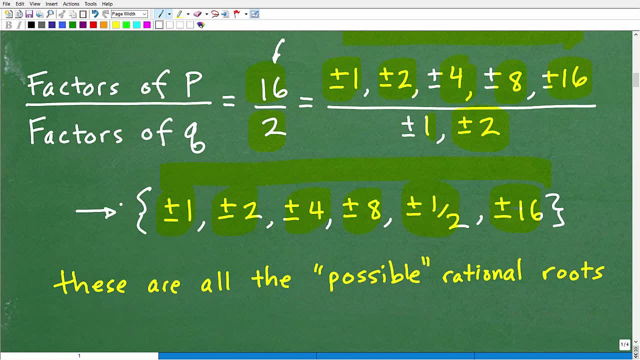 This is very important. That's where students get confused. But what does this mean? Well, if this polynomial that we're looking at, OK, has any rational roots, it's one of these guys. OK, it's within this set. 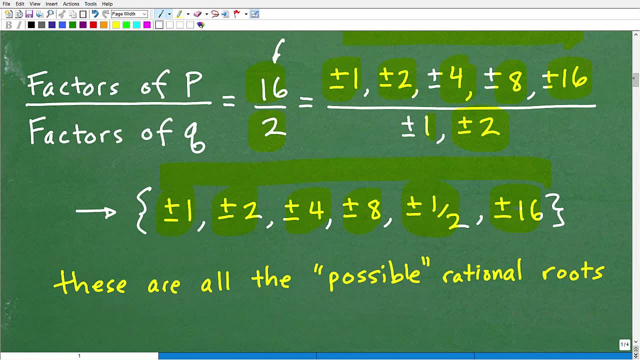 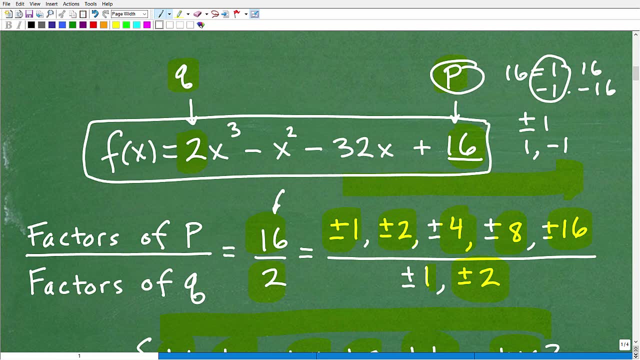 So these are all the possible rational roots. There's no guarantee, OK, there's no absolute certainty that this polynomial function, OK, has rational roots. We just don't know. I do know that it has three roots. OK, that could be real or imaginary. 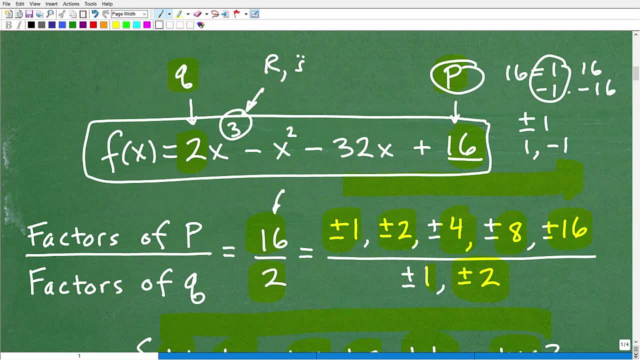 And there's other theorems and things that can help us out with this, But the rational root theorem is just one theorem, a part of other things that you need to, rules and techniques that you need to know, but very, very important. 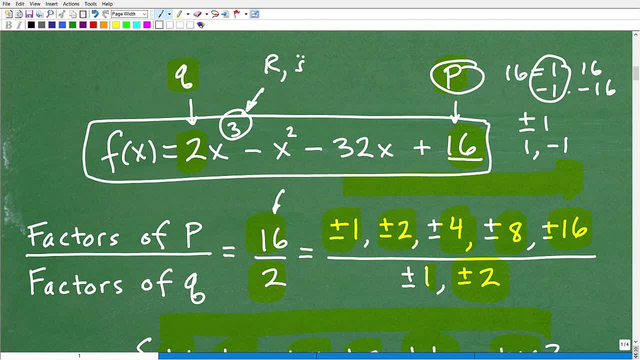 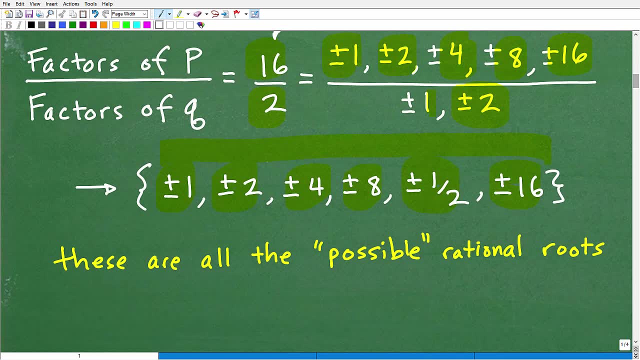 So we're like: OK, so if this polynomial equation has rational roots, it's going to be found with these guys, All right. So what do we do? Well, is that all of it? No, We want to now do what? 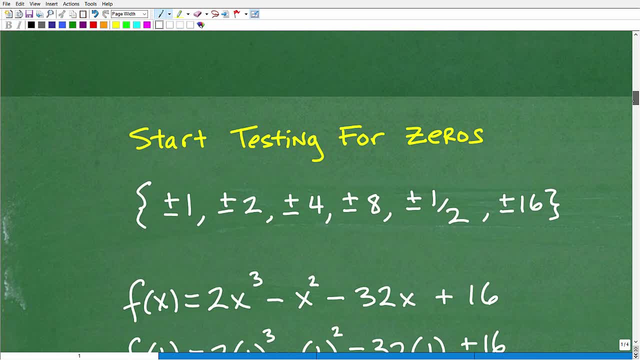 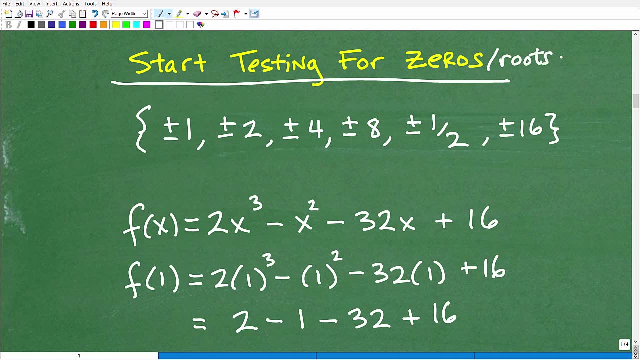 Well, let's go test these guys. Let's see if we actually have any rational roots. So let's start testing for zeros. Zero is another word for roots Or solutions. OK, so basically answers right. We're looking for the solutions to this equation. 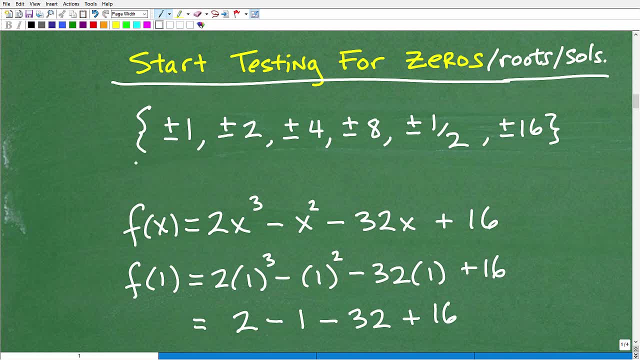 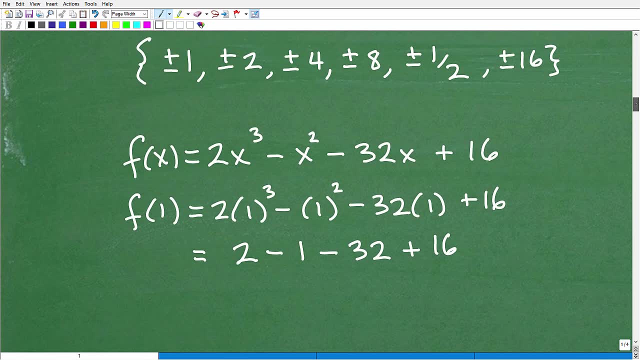 So here is our list of that. we just created all our possible rational roots. So how do we start testing for zeros? OK, it's pretty straightforward. There's two ways you can do this, and I'm going to show you the more common way here in a second. 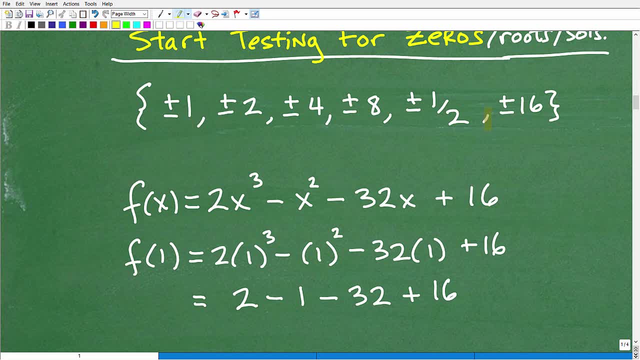 But if we have a solution, what we're really looking for. let's take: here We have positive, Negative one, So this means obviously one and negative one. Let's test for one. Let's start with the easiest number first. So if I plug in one into my function, 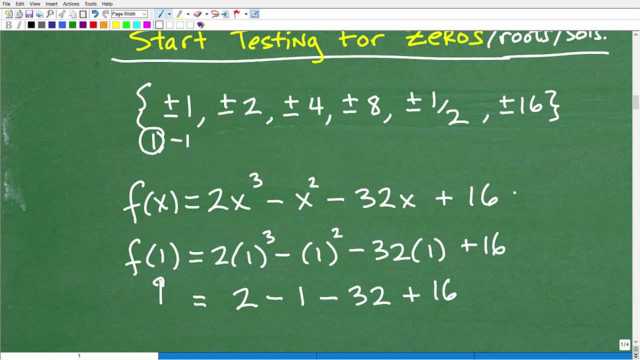 if I evaluate this function for one. all right, let's say, let me go over here. If I plug in and I'm looking for f of one and it turns out that that is zero, OK, if f of one equals to zero, then one is in fact a solution to this polynomial. 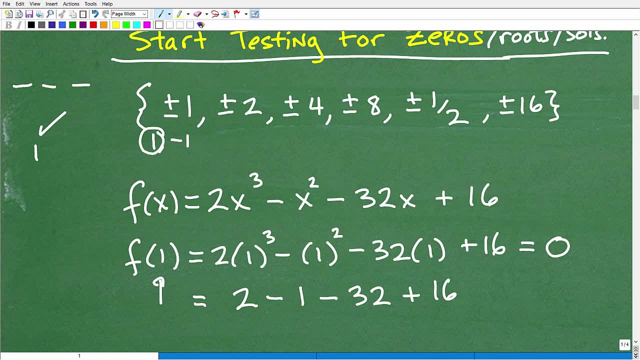 Then I need to find- Remember, I need to find three: one, two, three solutions. So hopefully they're going to be a part of this list. If they're not, then we've got to do other things Right. So the way we start testing is we can plug in these values. 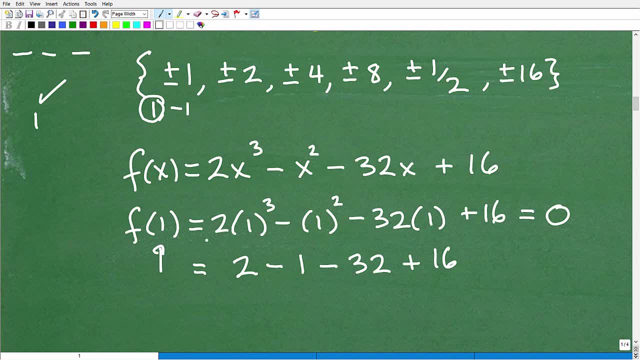 So like, for example, let's plug in one And when I plug in one into my function here you can see when I evaluate this one cubed that's going to be one times two. So you can see one squared is one. 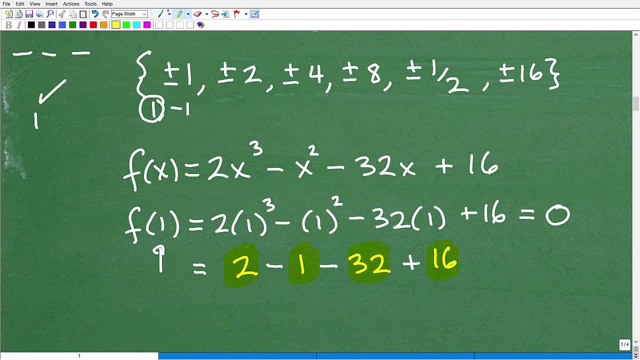 Thirty two times one is thirty two. Then you just look here. By the way, all this right here is going to add up to zero, OK, meaning that one is not a solution. So well, you know, I'm not going to be sad about it. 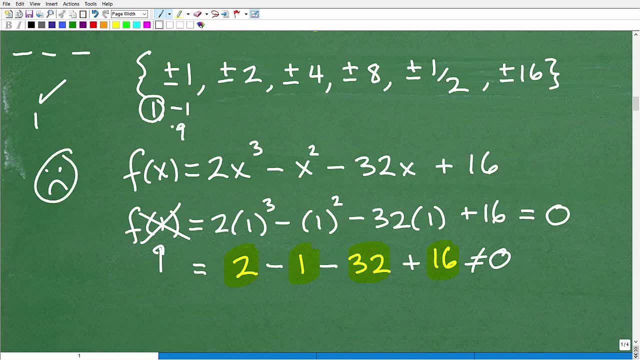 I got a lot of other good numbers here to test, Right. So then I would move on and test negative one, And then I would you know. if that didn't work, OK now, if it did work, now that's a whole nother discussion. 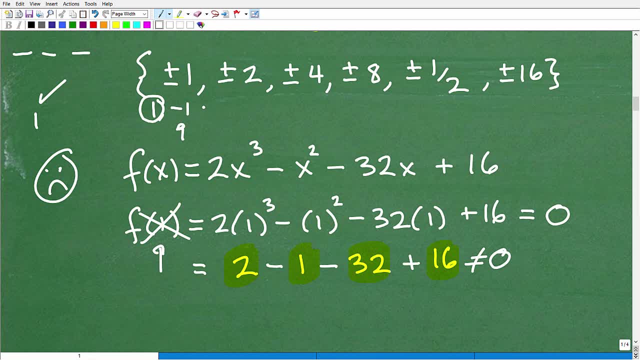 OK, so I'm really focusing in on the rational root theorem. There's- this is part of the broader topic of solving higher order polynomial equations- But let's just kind of stick to the application of the rational root theorem. OK, so I could just keep testing these numbers. 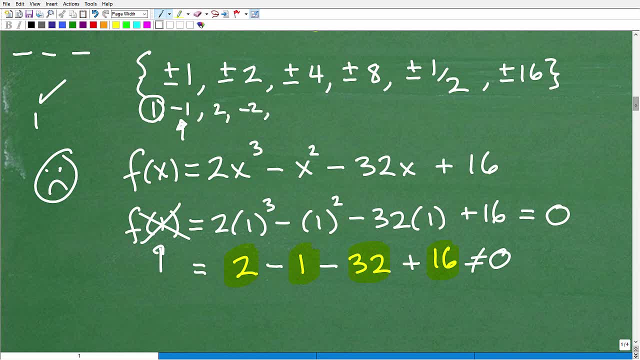 I could test two negative, two, four. I'm just looking for rational roots Now. you can do it this way, but that's not the way your teacher is likely going to want you to approach it. OK, so we know one is not positive. 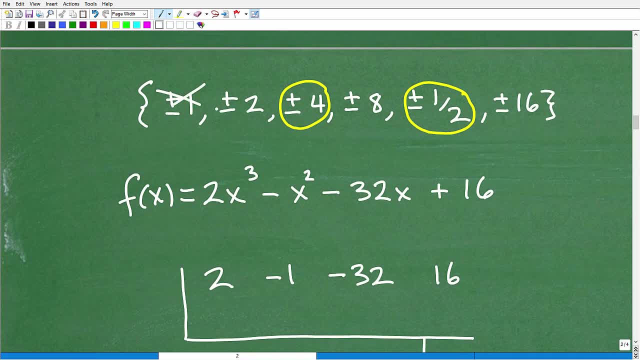 One is not an answer, So we would go through this list. Now you can see here I'm highlighting values, rational numbers that are, in fact, our solutions to this polynomial equation. OK, now let's go ahead and take a look at what I'm doing here. 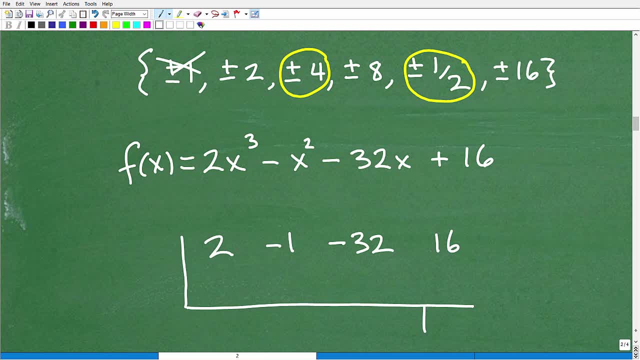 This is called synthetic division. You need to be familiar with this. OK, hopefully you know how to use synthetic division. This is how it works. OK, so you can see my coefficients here: two negative one. So I have x squared negative 32, and then I have 16.. 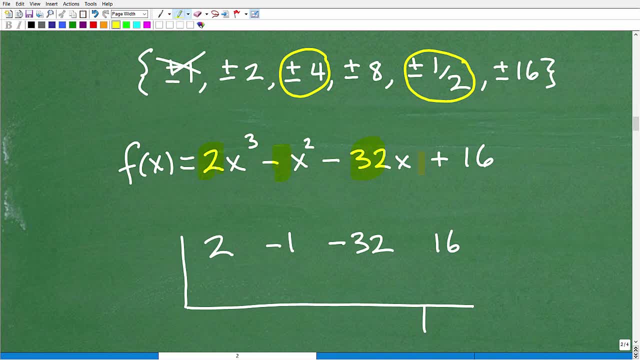 So using these coefficients here? OK, I'm going to plug them down here, like so. OK, if you don't understand synthetic divisions, check, check, check out my video on the remainder theorem. I'm going to make a dedicated video on polynomial division and synthetic division. 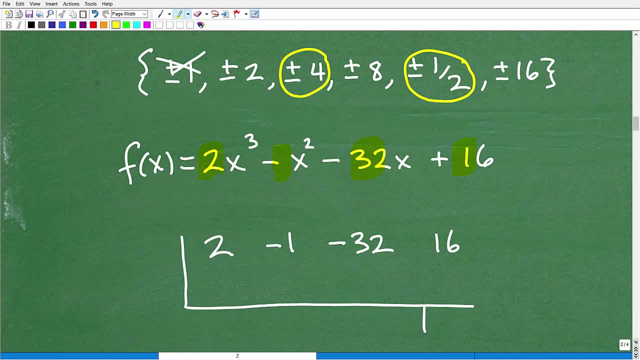 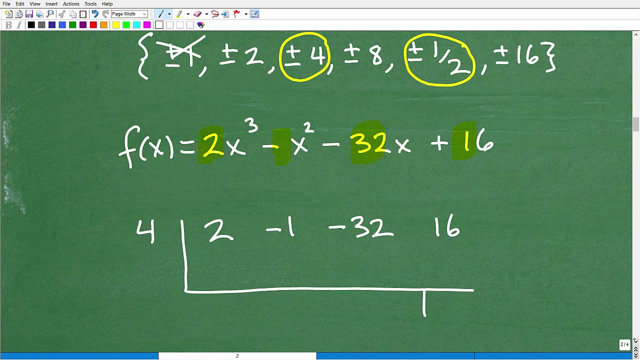 So that may already be like in my Algebra 2 playlist, But this is what you need to kind of structure, OK, so let's go ahead And test positive for OK, how does this work? Well, again, I'm assuming that you may know a little bit about synthetic division. 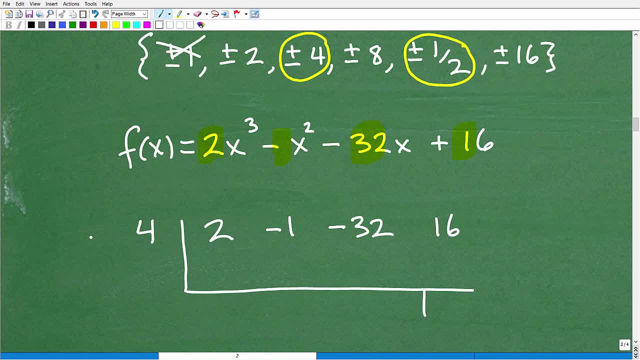 It's really really cool technique And this is the easier way to evaluate or to test for zeros. OK, so you see this little two right here. this two first step is once we get this all written correctly and we do this little L thing just like this. 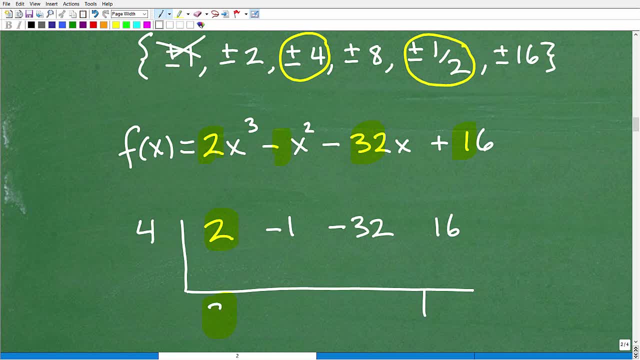 you make it just like this. we're going to drop that number right there. OK, boop, Now we're going to go four times two is what That's eight? OK, so negative one, And we're going to add down: plus eight is seven. 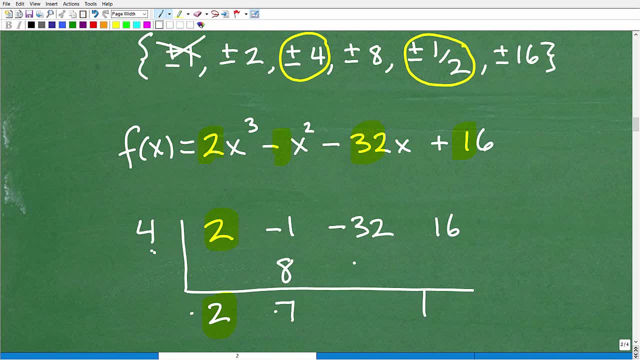 OK, now we're going to go four times seven is what Twenty eight? Then we're going to add down negative thirty two plus twenty eight is negative four. OK, so make sure you understand what I'm doing. I'm adding down. Now I'm just going to continue the pattern. 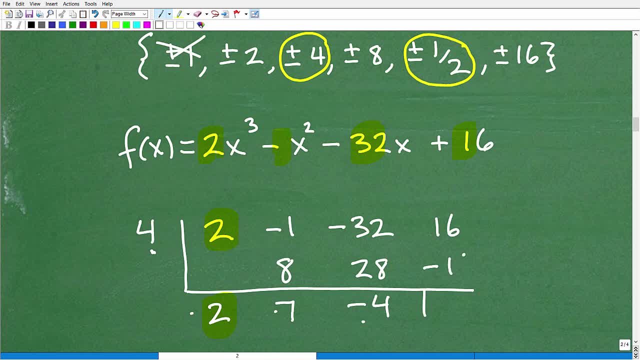 Four times negative four is what Negative sixteen, And when I add down here this is my remainder, It is zero. OK, meaning that if I was to plug this into this function f of four, into all of this stuff, I would get zero. 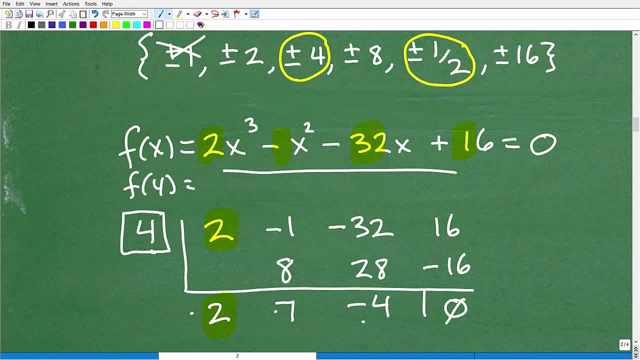 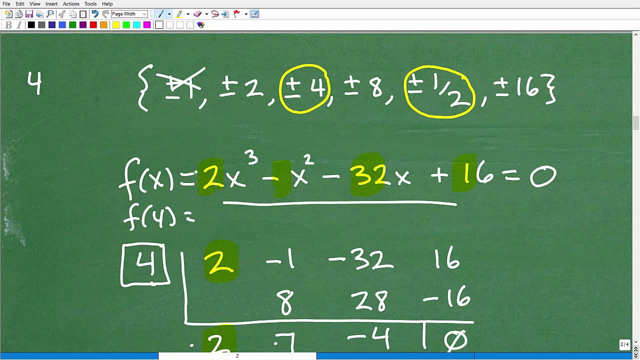 OK, so that's an indicator, that is validation, That four is in fact a solution to this polynomial equation. OK, If you keep testing, you'll see that negative four is one as well, And then either positive or negative one half, I can't remember which one is. 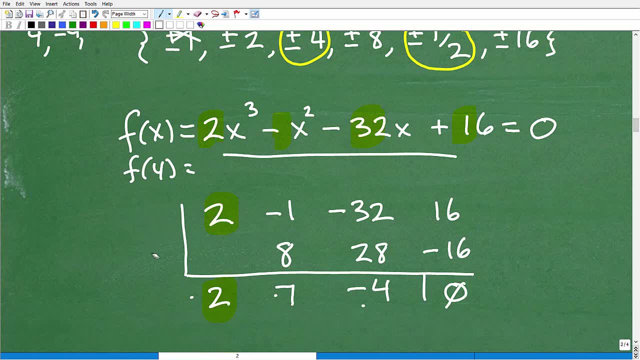 But we can go ahead and actually let's test for positive one half real quick, just to kind of reinforce how this stuff works. OK, I think it's positive one half. I already did this problem in advance, but let's put one half right here. 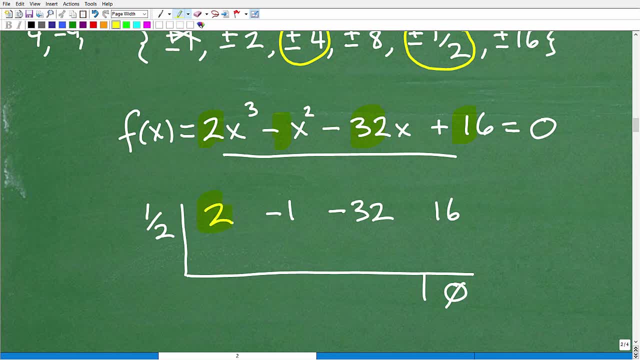 Let's test for one half OK. so again, you're going to take this first number drop down there. I don't know if that's zero, OK. so two times one half OK is one negative one plus one zero one half times. 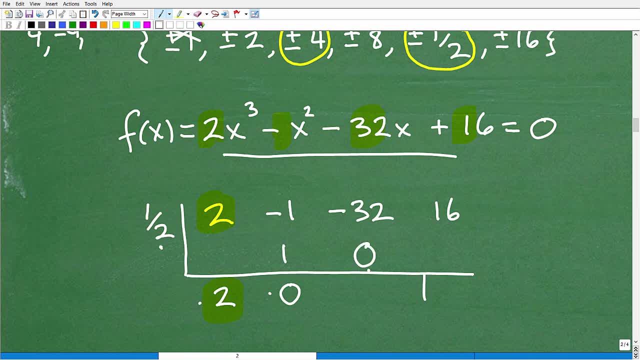 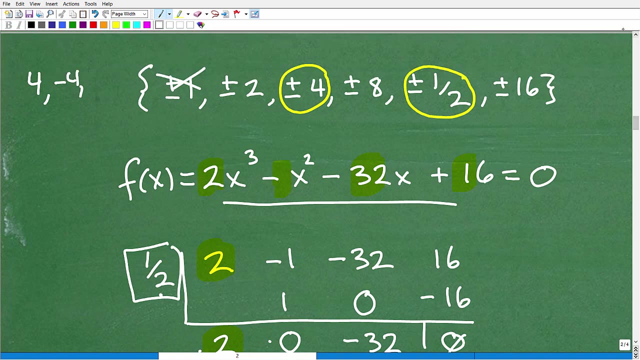 zero, zero, negative. thirty two plus zero is negative. thirty two, one half times negative. thirty two negative sixteen- Look how awesome this is: Sixteen plus negative, sixteen is zero. So here we have one half and we have our positive, negative four. So one, two, three solutions to my third degree polynomial. 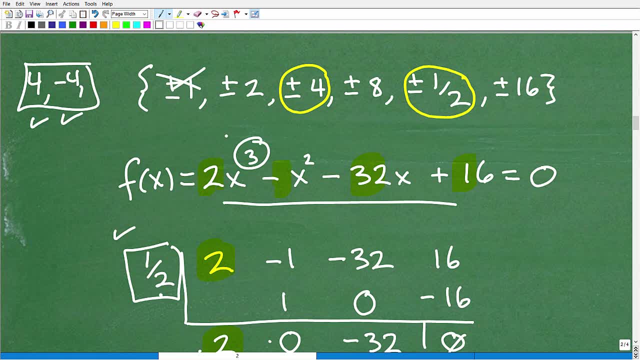 I am all done. They happen to be all rational roots, but there's no guarantees. OK, so again, a rational root theorem says: listen, if this thing does have rational roots, it's going to be amongst this whole list that you create with these factors. 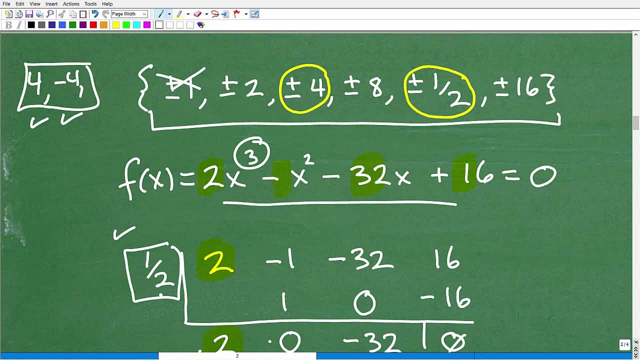 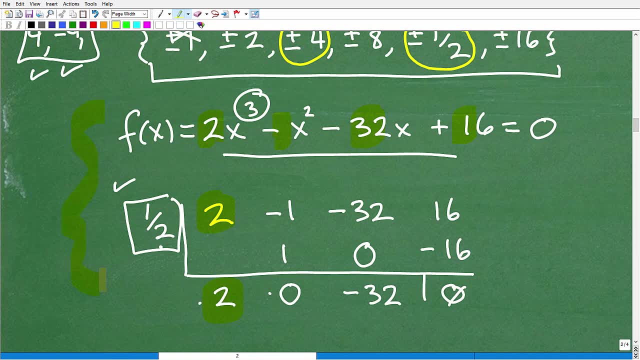 of P's and Q's Very, very, very important theorem indeed, And of course, you know there's a lot involved here and I can keep going on and on. That's why I really need to, you know, look at. 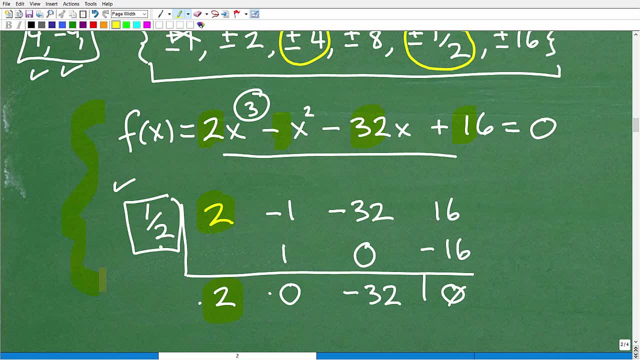 additional YouTube videos that I've made. But if you really want to master this stuff, you got to maybe jump into my algebra, two course. OK, I really get into this because other techniques we want to consider. We want to be looking at graphs and the demorphs theorem, not demorphs theorem. 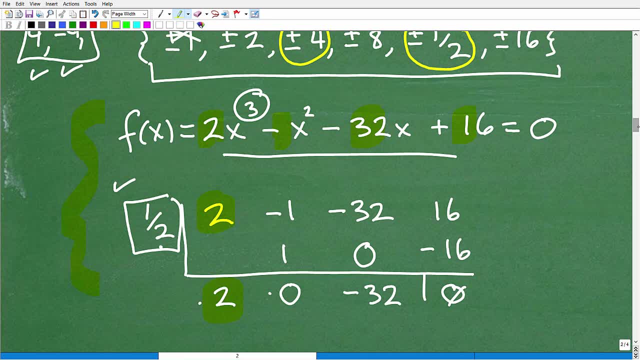 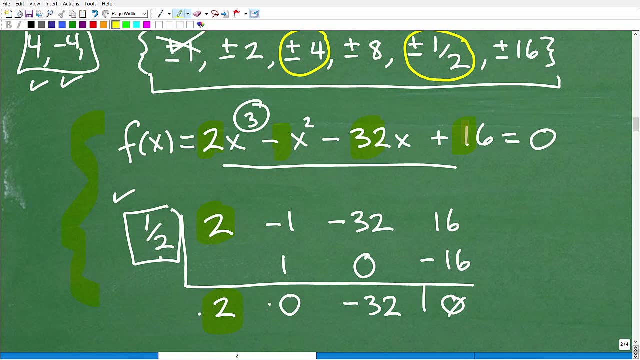 Descartes rule of signs. There's other things here that can help us solve. because let's suppose that we didn't have any rational roots. Let's say we didn't find we test all these guys and we didn't have any rational roots. We would be very sad because we were like: what do we do now?